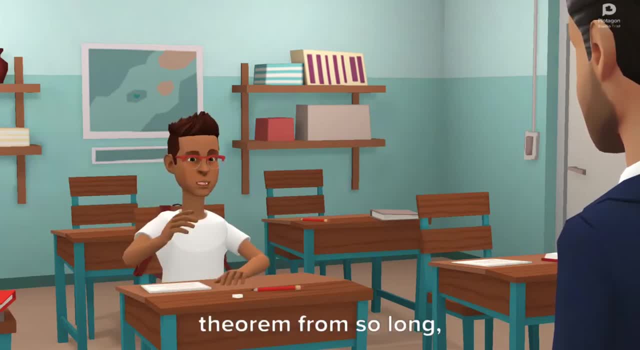 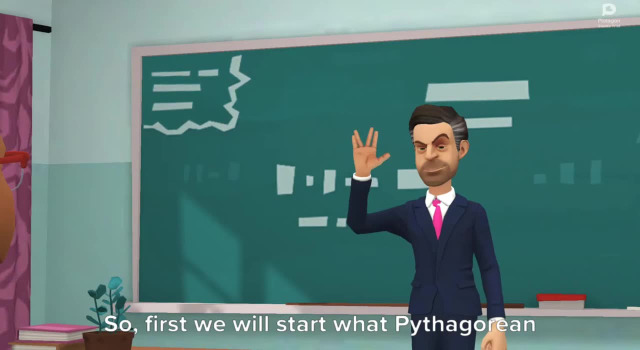 Hi Teacher. We are learning about Pythagorean Theorem from so long. What are its uses? This is a very good question, So first we will start with Pythagorean Theorem is. The Pythagorean Theorem states that the sum of the squares of the legs of a right triangle 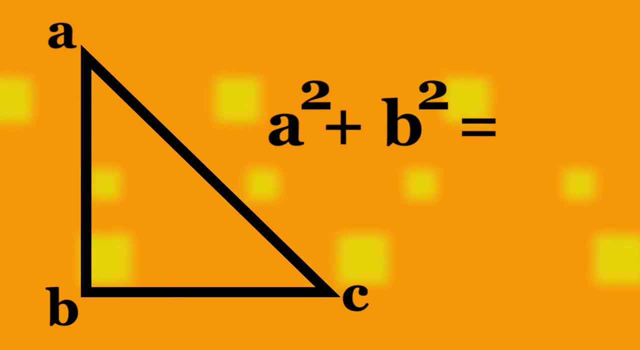 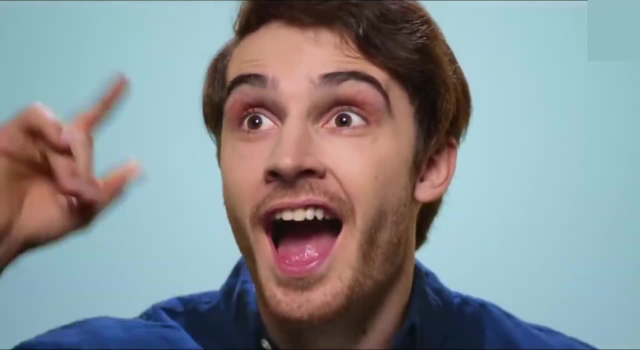 that is a square plus b square, is the same as the square of its hypotenuse, that is c square. Now let's see where we are actually using it in real life. The Pythagorean Theorem can be used in numerous ways, for example, even on a baseball stadium, Since the bases 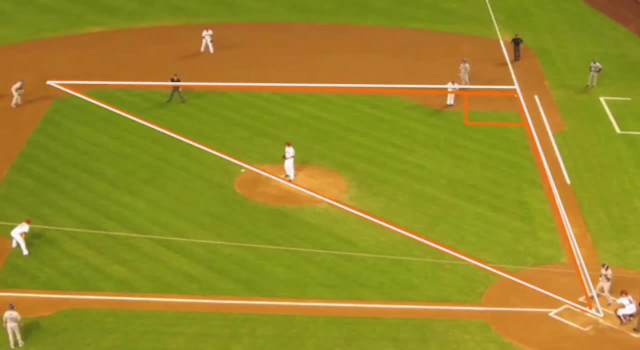 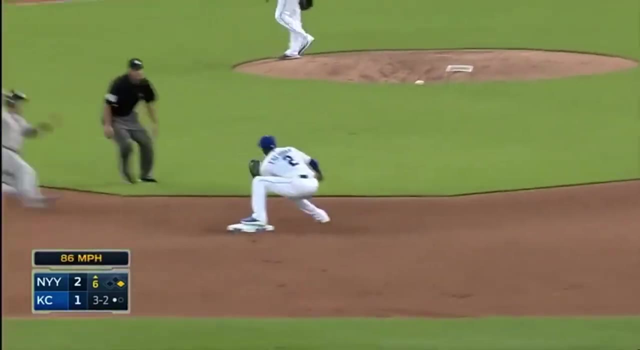 are each 90 feet apart in the form of a square. the theorem helps us to find the distance the catcher has to throw the ball to get to second base when a runner is trying to steal, The right triangle formed would be with half of the infield where the legs of the triangle 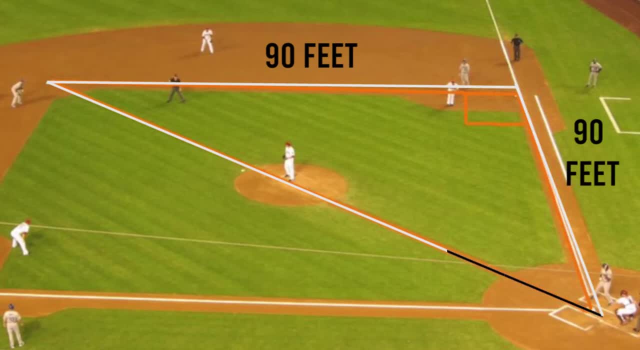 are the base parts of 90 feet each and the hypotenuse is from the home plate to second base. The hypotenuse can be found by looking at the diagram on the left hand side. If we look at the diagram on the right hand side, we can see that the hypotenuse is from the base. 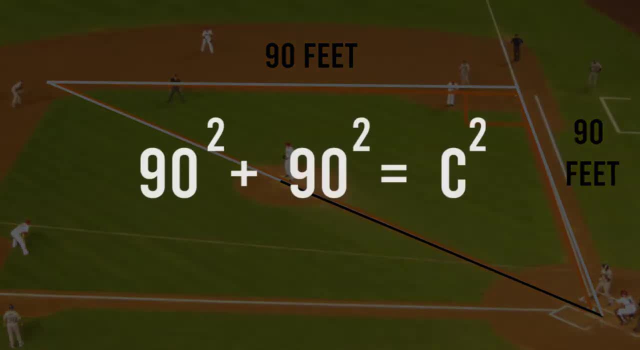 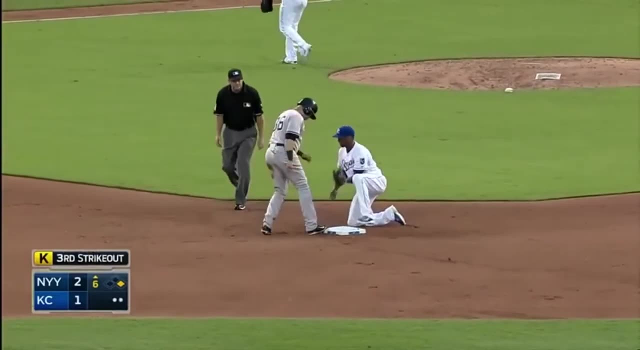 solving the equation: 90 square plus 90 square equals c square. that is, solving c will show us that the throw is about 127.3 feet. this information is useful because it will give the coaches an idea about how hard the catcher needs to be able to throw a ball accurately in order to throw a. 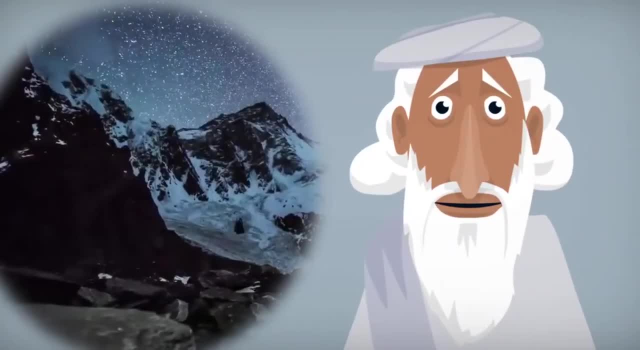 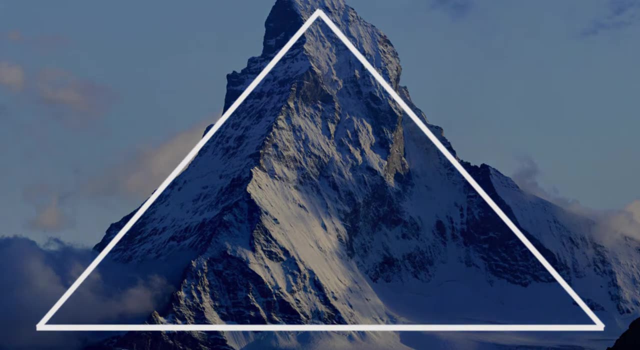 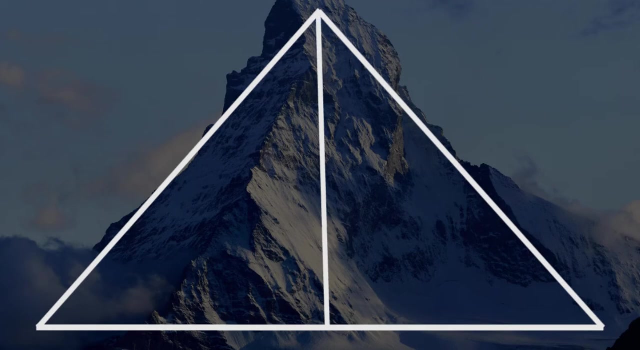 runner out. pythagoras theorem can also be used even in the case of mountains. the horizontal and vertical distances from the foot of the mountain to its top can be determined on a map forming the legs of a right triangle that can be drawn in the mountain center, the third side of the triangle. 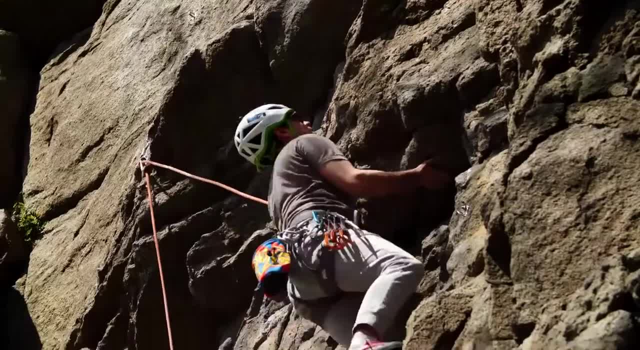 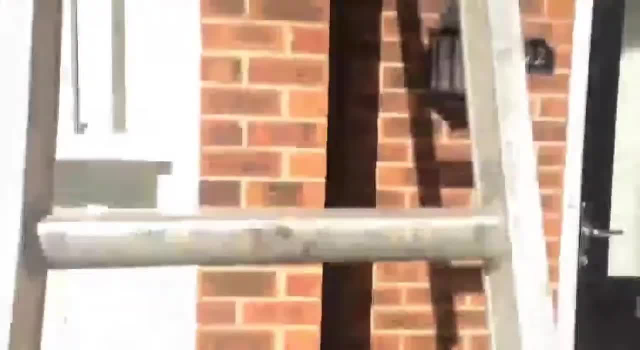 the hypotenuse represents the walk of the mountain, which never has to be physically measured, since it can be found using the pythagorean theorem. painters use ladders to paint on high buildings and often use the help of pythagoras theorem to complete their work. the painter needs to determine: 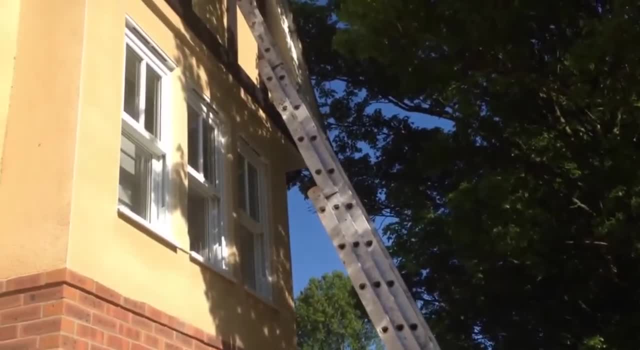 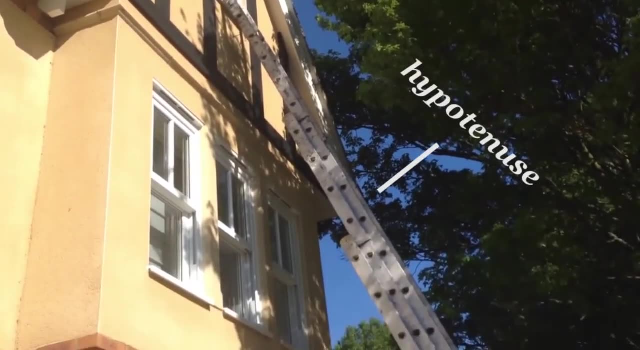 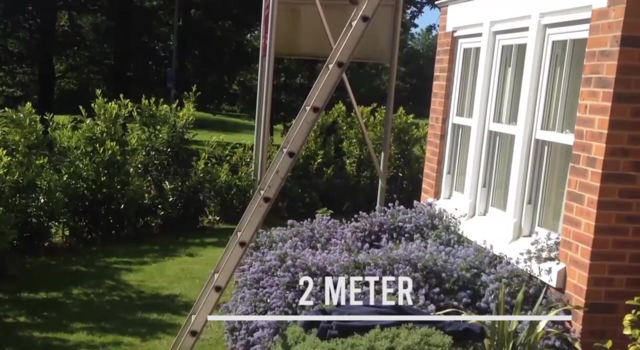 how tall a ladder he needs to be in order to safely place the base away from the wall so it won't tip over. in this case, the ladder itself will be the hypotenuse. the painter has to put the base of the ladder two meter away from the wall to ensure it won't tip. what will be the length of? 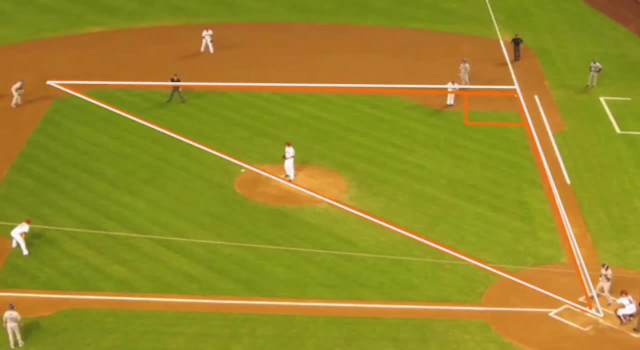 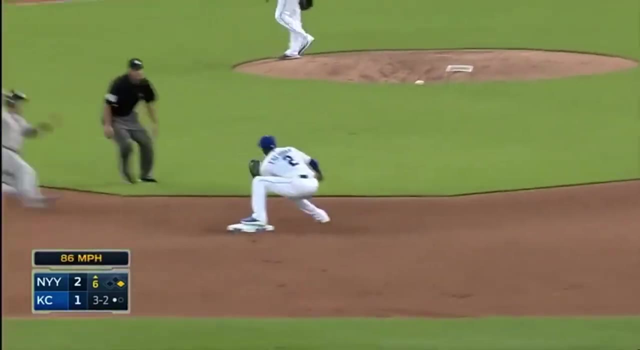 are each 90 feet apart in the form of a square. the theorem helps us to find the distance the catcher has to throw the ball to get to second base when a runner is trying to steal, The right triangle formed would be with half of the infield where the legs of the triangle 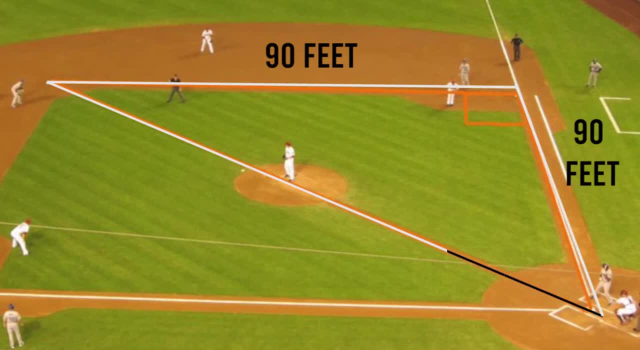 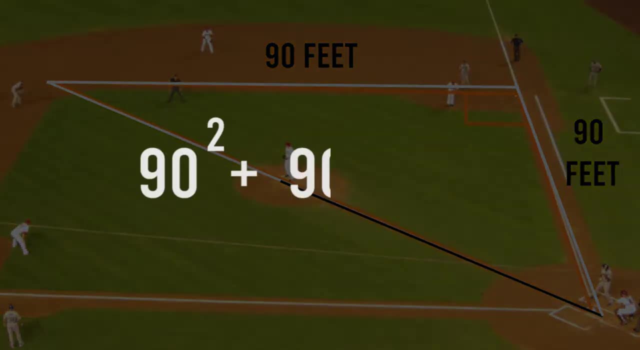 are the base parts of 90 feet each and the hypotenuse is from the home plate to second base. The hypotenuse can be found by solving the equation: 90 square plus 90 square equals c square. that is, solving c will show. 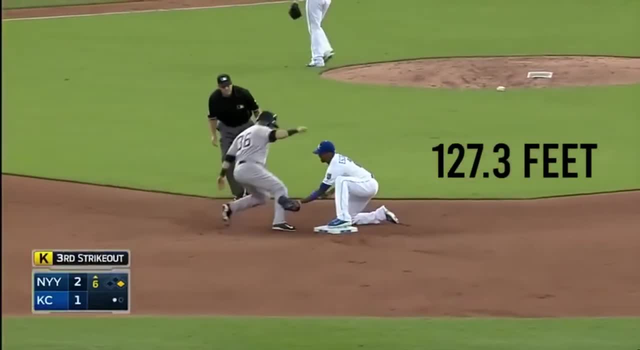 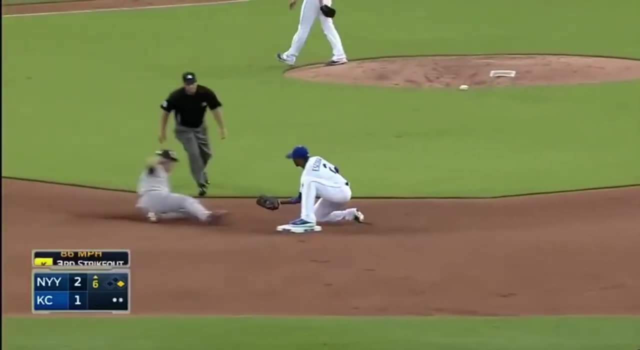 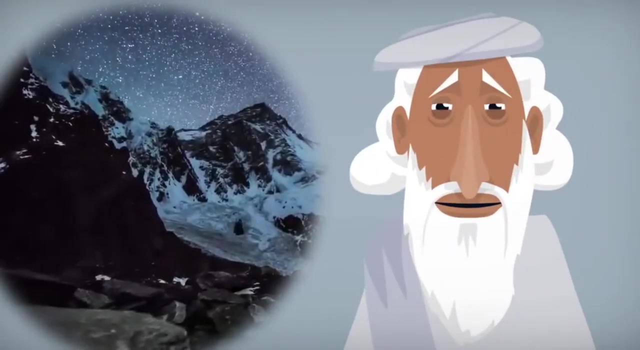 us that the throw is about 127.3 feet. This information is useful because it will give the coaches an idea about how hard the catcher needs to be able to throw a ball accurately in order to throw a runner out. Pythagorean Theorem can also be used even in the case. 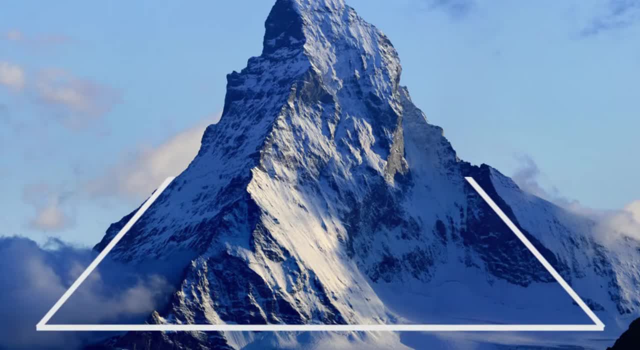 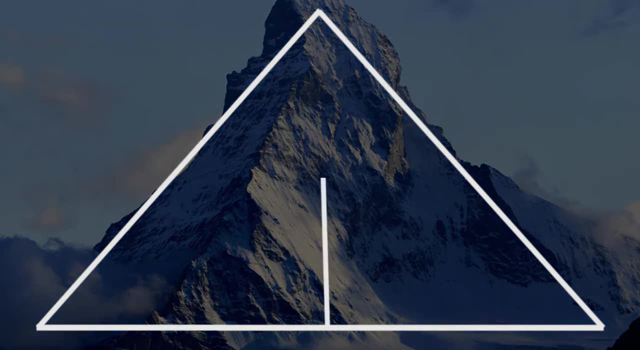 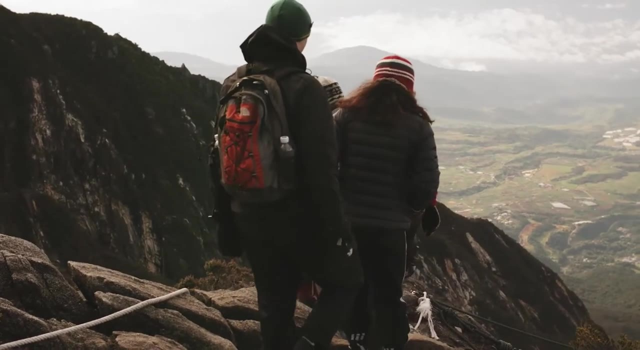 of mountains. The horizontal and vertical distances from the foot of the mountain to top of a mountain can be determined on a map forming the legs of a right triangle that can be drawn in the mountain's centre. The third side of the triangle, the hypotenuse, represents the walk of the mountain, which 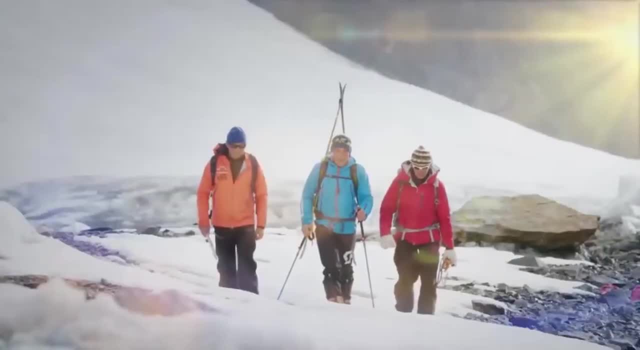 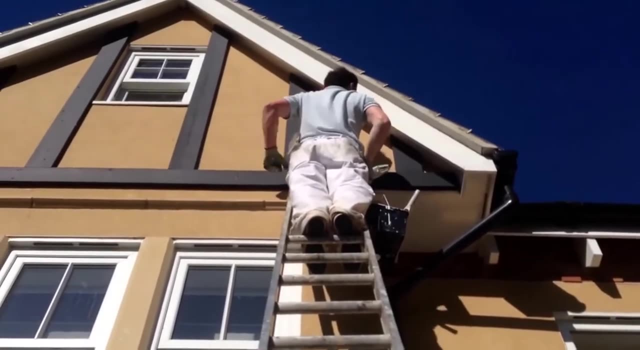 never has to be physically measured, since it can be found using the Pythagorean theorem. Painters use ladders to paint on high buildings and often use the help of Pythagorean theorem to complete their work. The painter needs to determine how tall a ladder he needs to 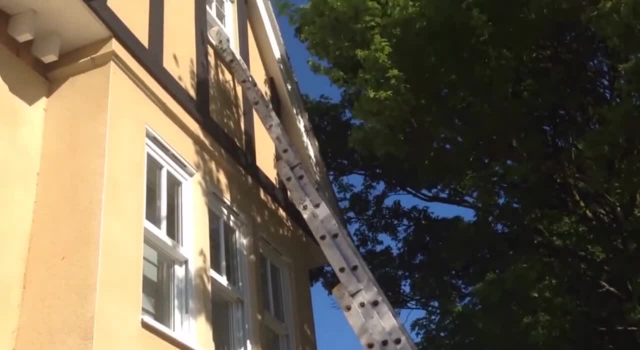 be. in order to safely paint on high buildings, The top of the ladder is the height of the Pithagorean Theorem. place the base away from the wall so it won't tip over. In this case, the ladder itself will be the hypotenuse. 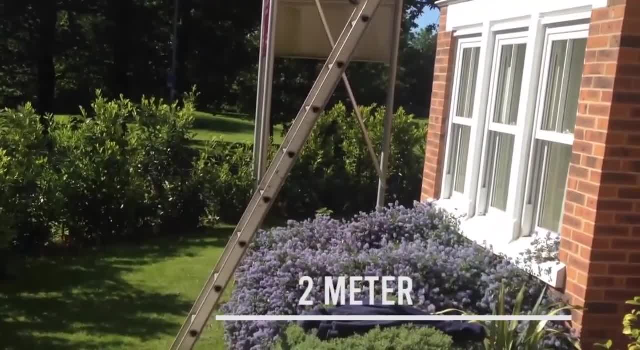 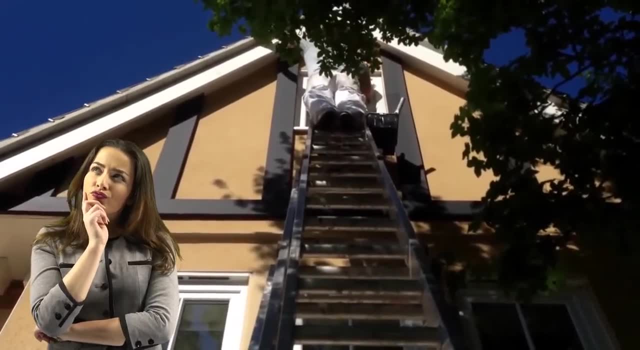 The painter has to put the base of the ladder 2 meter away from the wall to ensure it won't tip. What will be the length of the ladder required by the painter to complete his work? You can calculate it using Pythagoras theorem. 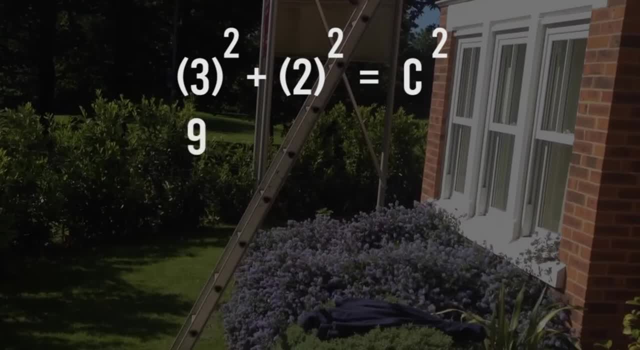 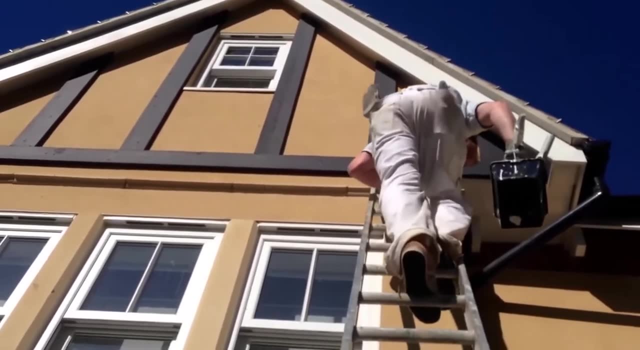 3 square plus 2 square is equal to c square, that is, 9 plus 4 equal to c square. So root 13 equal to 6, that is 3.6 meters. Thus the painter will need a ladder at least about 3.6 meters high.